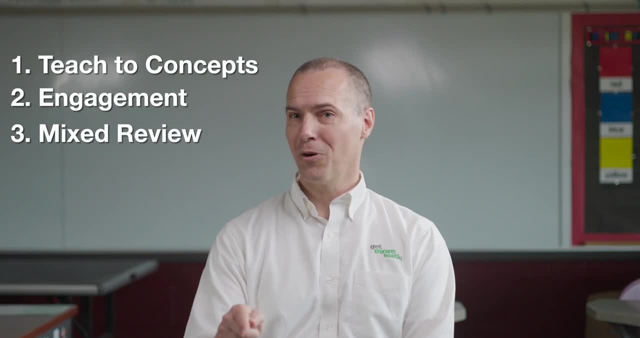 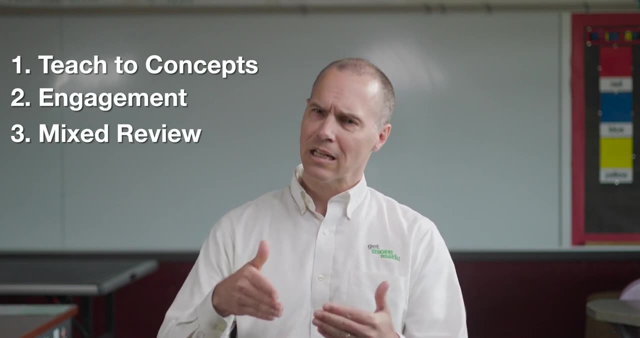 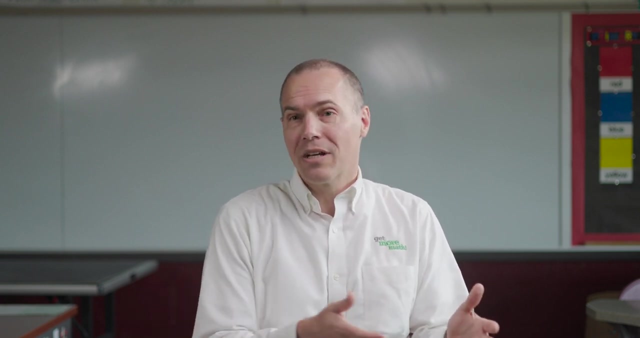 And that's why I wrote Get More Math, that third piece. You know, as a teacher I could find ways to get kids engaged. I could really seek to connect to concepts. I could build a powerful curriculum, and I did, but I could still get to the end of the school year and discover that everything had sort of faded away. 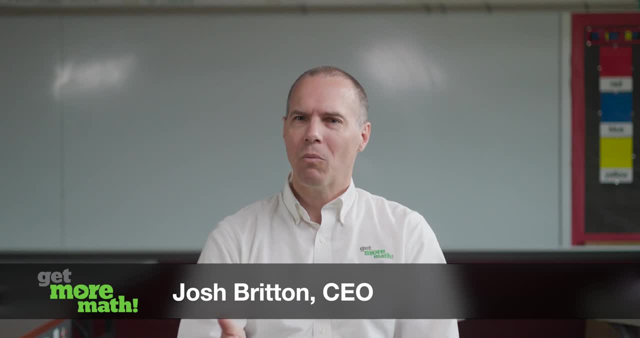 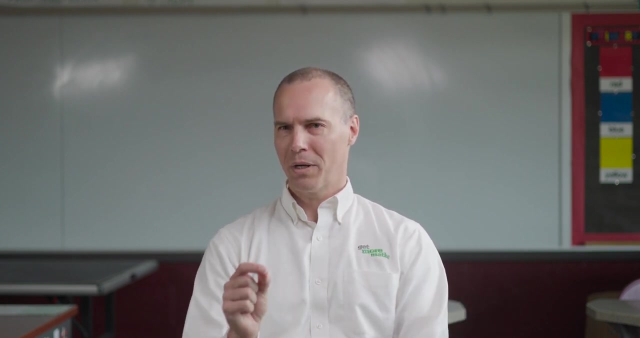 So the question is: why does that happen, And why does that happen in such a widespread fashion, like across the United States? Everybody I talk to says, oh yeah, I forgot everything I learned in algebra. Well, why? Of course, there are many reasons, But one one in particular that I want to focus on is how people use their time, how teachers invest themselves and their minutes in a typical classroom. So, generally speaking, the pattern in an American classroom is: let's have a lesson on new content and then let's practice that content. In my view, there's a pattern in an American classroom. 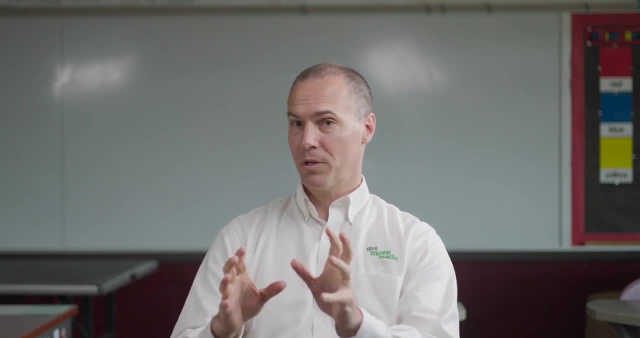 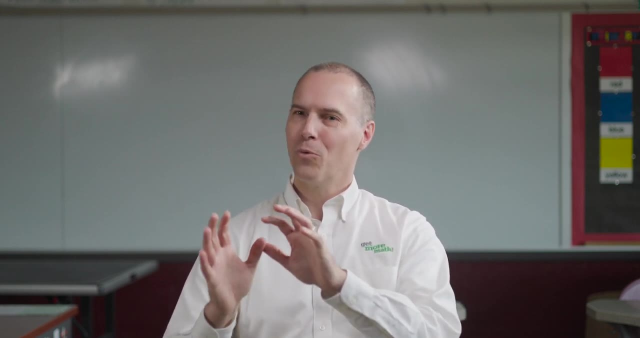 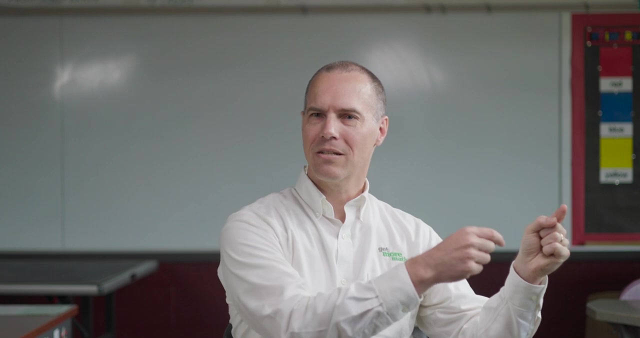 So there's a piece that's missing there. To really get to it, let's just think about what's happening. Day one: let's learn a new thing, practice it some. Day two: learn a new thing, practice it some. Repeat process, take a unit, test, start another unit. New thing, new thing, new thing, practice, practice, practice. 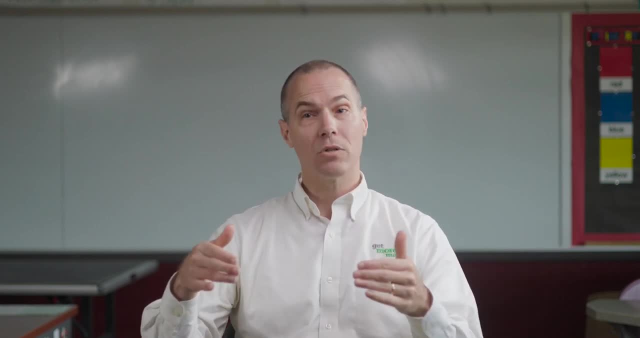 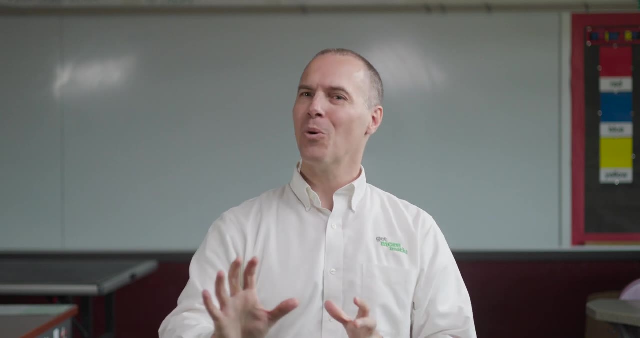 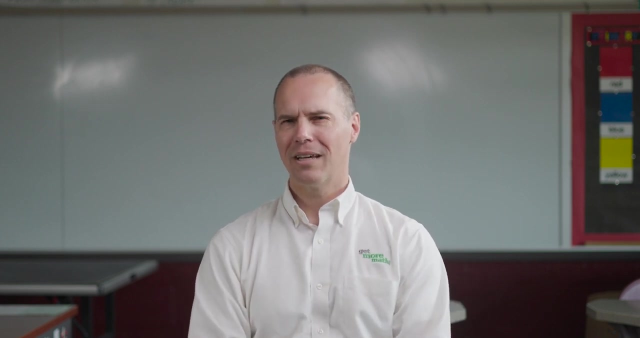 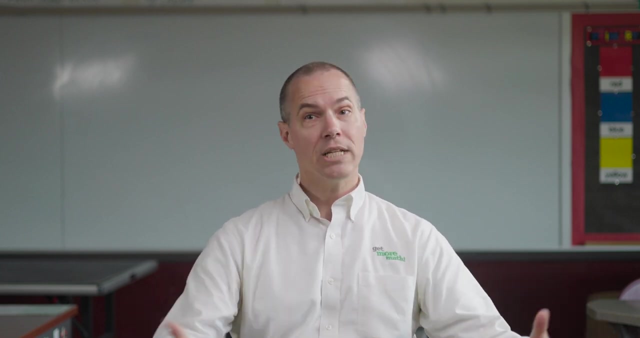 Perhaps we mix in a little bit of maybe in warm-ups, some reach-back reviews, some spiral review, But the dominant emphasis is move forward, conquer new territory. Unfortunately, that's not a very brain-friendly approach. It's odd to me. We all know that Nobody hears me say this and says no, no, no. Kids, if they learn 180 lessons back to back to back to back, retain everything. 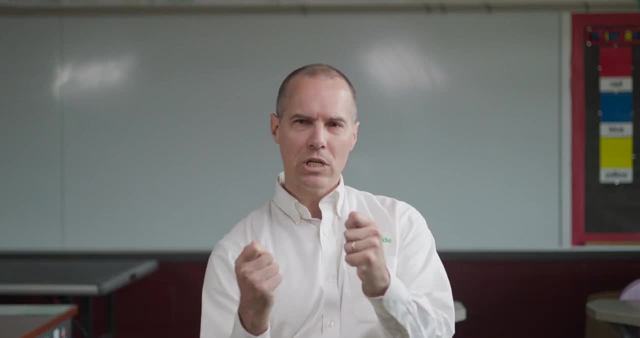 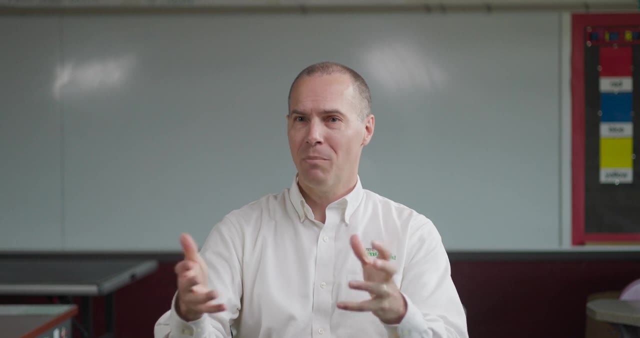 And yet the effort that it takes to retool your approach, how you invest minutes, is significant and perhaps even it seems too big of a barrier. It's not. I'm telling you, you can do it, I did it. 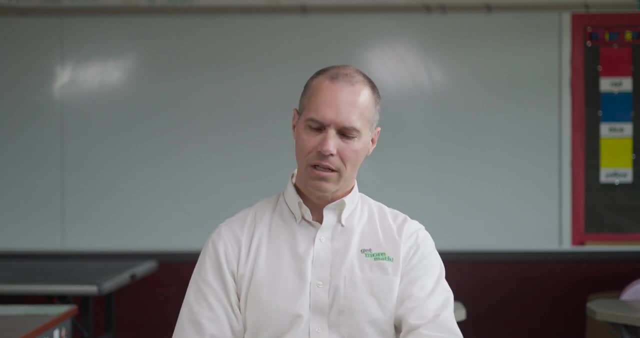 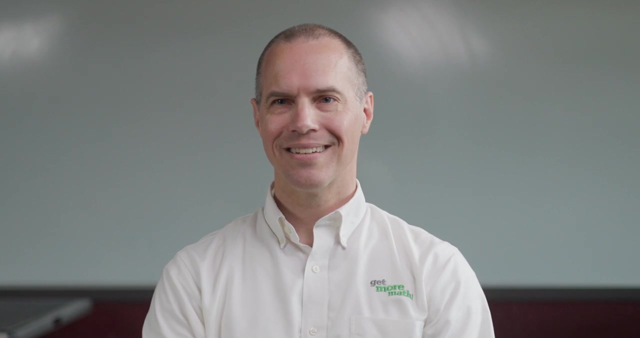 And it made a huge difference when, instead of just teaching a new thing and practicing it, I added a third component, That is to say, I invested in mixed review every day. Get More Math provides daily sessions of cumulative mixed review, Individualized to each student's needs.